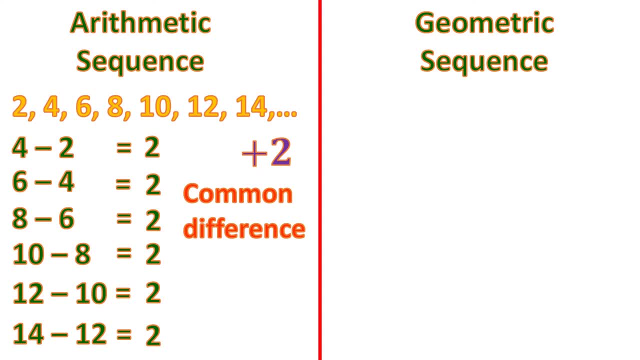 addition, it's adding two, but it's called common difference because you can get the the two by subtracting four minus two, or the second term minus the first term. that's why it's called common difference. so the common difference is denoted by D, which is equal to the. 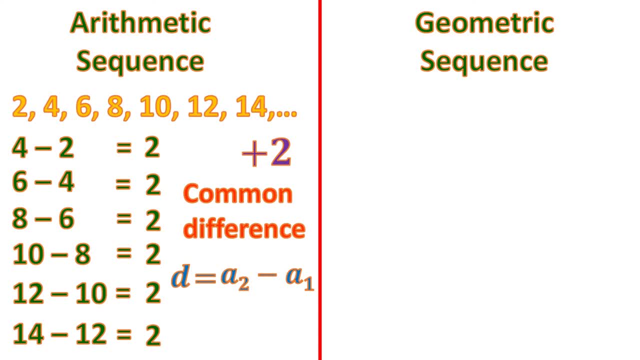 second term minus the first term. but this formula is not general, it's just specific, that second minus the first. but actually you can do it to the rest of the terms. you can do third term minus the second term and so on. so that is common difference. now for the geometric sequence. let's have this: 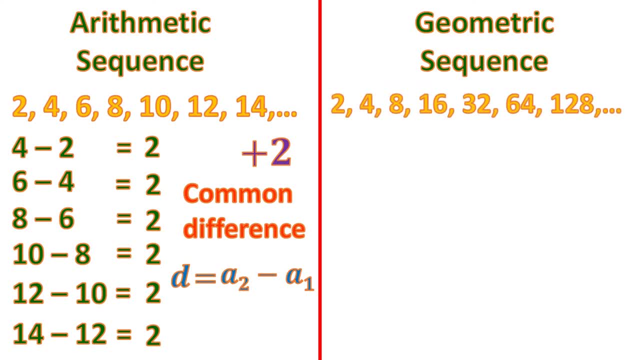 example of sequence 2, 4, 8, 16, 32, 64, 128, and so on. and so let's um. how will you know that this is geometric sequence? when you times, uh, a number and you will generate this sequence. so, in this case, you times it with two. two times two is four, four times two is eight, eight times two. 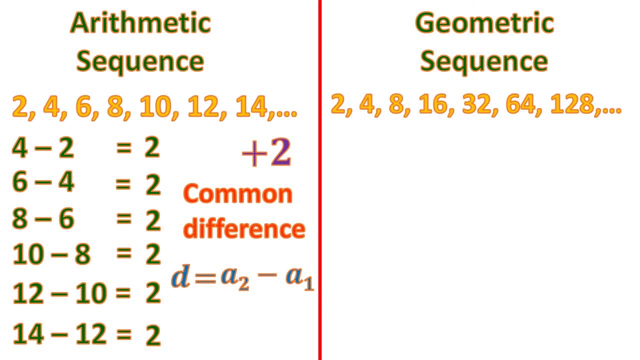 sixteen, sixteen times this thirty two, thirty two times to sixty four, sixty four times this one today. and so that means it is a geometric sequence, because we have a common number that is multiplied to generate a pattern. so if you, if you divide four by two, or any number by divided by before that, 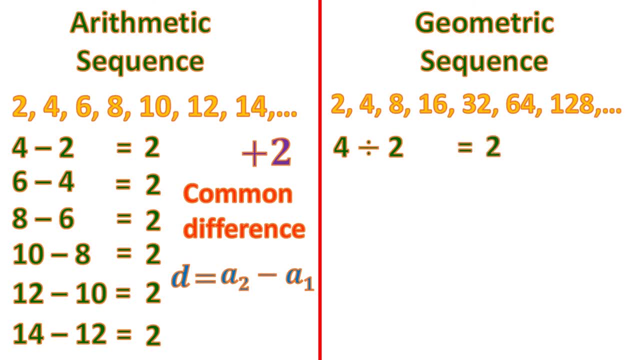 it will be um. it must be the same. so it's equal to two. eight divided by four is two. 16 divided by 8 is 2, 32 divided by 16 is 2, 64 divided by 32 is 2, and 128 divided by 64 is 2. 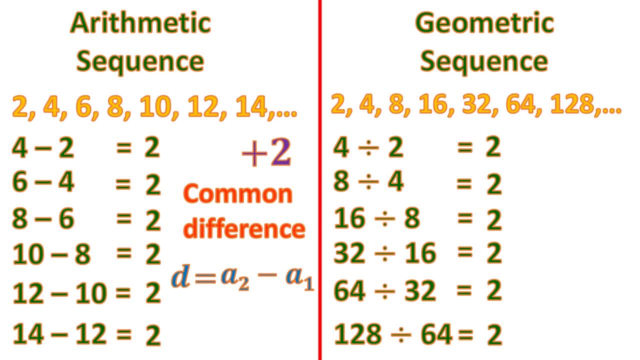 so that 2 must be the same, so that it will be a geometric sequence. so to generate the sequence, you multiply by 2 and this is what you call the common ratio. so why a ratio? ratio is also means fraction. it's because so to get the rate common ratio, denoted by R, you divide the.